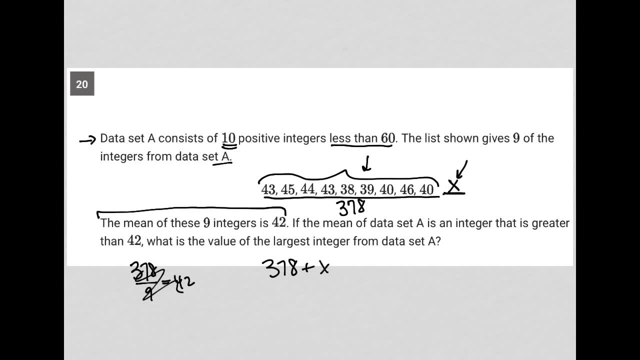 plus x from the missing 10th value. Now we're dividing by 10, because we have all 10 integers. So we can do this by adding up the 2 integers from data set A, and then we're being told that that must be. 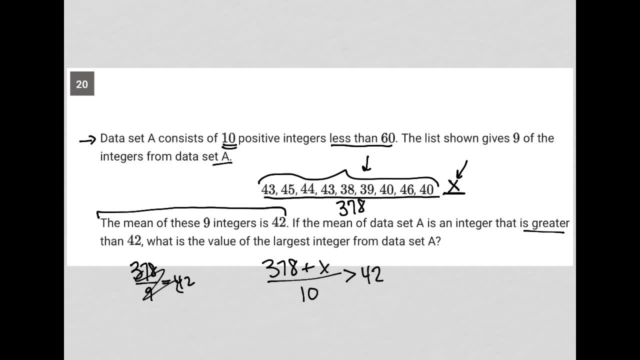 greater than 42.. And we're told that it's an integer right, which is important because that means it's not a decimal. Okay, so that's important. The question goes on to say: what is the value of the largest integer from data set A? Well, I can just simplify this inequality here by multiplying. both sides by 10, and I'd have 378 plus x is greater than 42. Now this equals the sum of the values that I have here, and I'm going to multiply both sides and that's the end result. So in this, 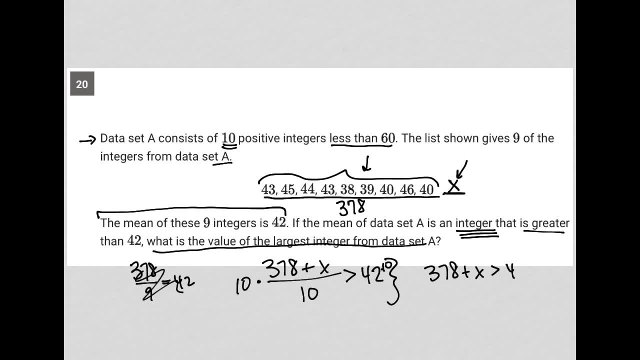 value here. I'm multiplying both sides by 10 and I'd have 378 plus x is greater than 42.. Now you can 420.. And I want to get the greatest value that x can be and still have x be or still have the. 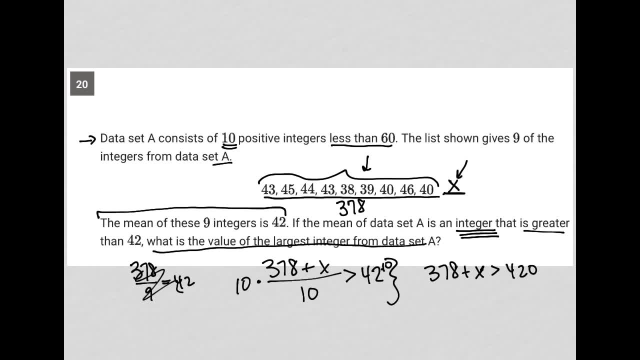 average be an integer. Now, how does the average remain an integer, right? So again, the mean for data set A is 378 plus x over 10.. So, whatever x is, I need to make sure that this numerator will still be a multiple of 10.. If I simplify what I have here: 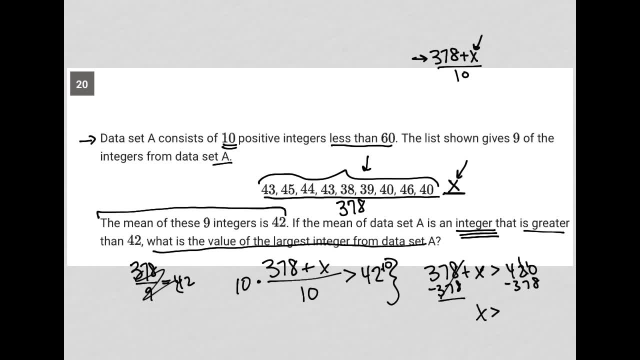 I'm getting. x must be greater than okay, x must be greater than 42. And so that's the minimum. 43 is like the minimum number it can be, since it has to be integers, But if I were to place 43 here, I need something that okay. 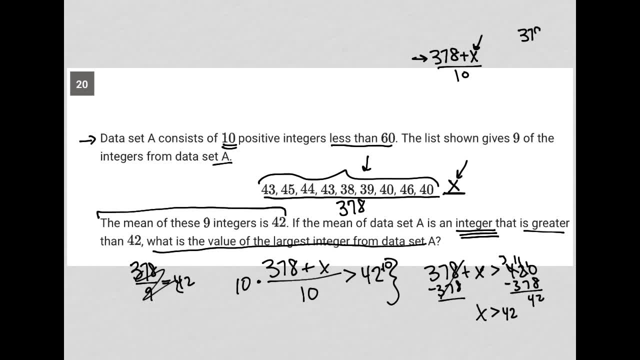 so here's the minimum, and I need something that's greater than 42.. And so that's the minimum. so here's the minimum, and I need something that's greater than 42.. And so that's the minimum. I know what's going on. I have 378.. I want my x value to, once added to 378, to be a multiple of 10.. 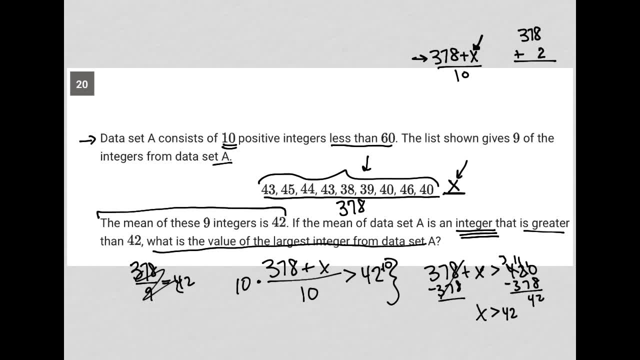 It means I need to have this number here, needs to be a two. There really isn't any other option, right? I need to make sure that when I add these two numbers together, that I have a zero at the end, And that's the only way that that's going to work out. So if I put 42 here, that should work. 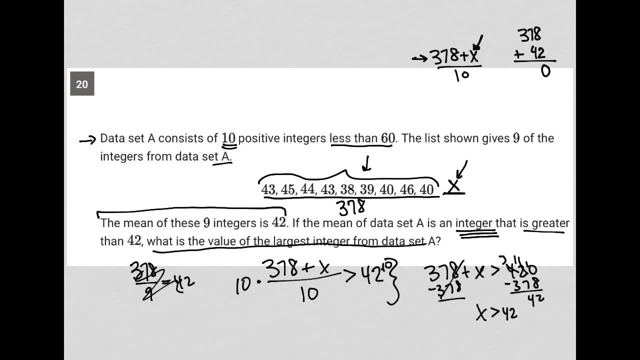 I'm not sure that's going to be the biggest number, but that should give me a value. But also, if I put 52 here, that's larger. In fact, that's why I can't use 42, because x has to be greater.